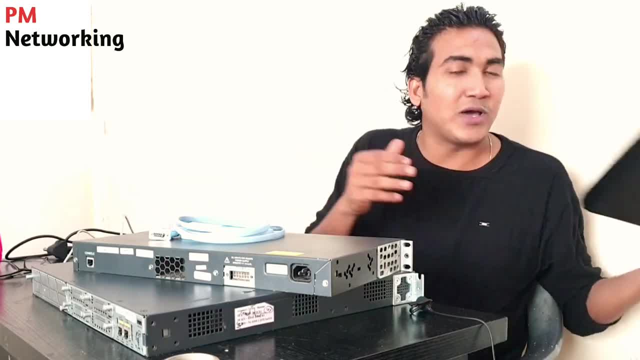 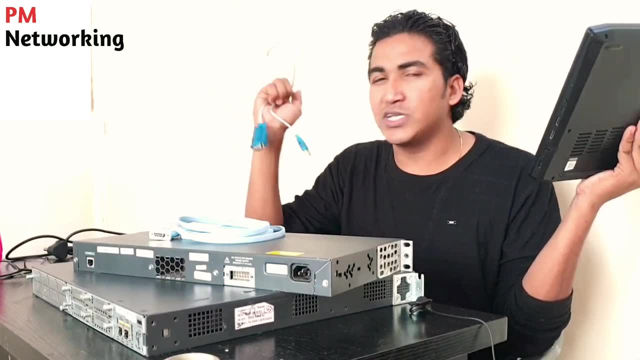 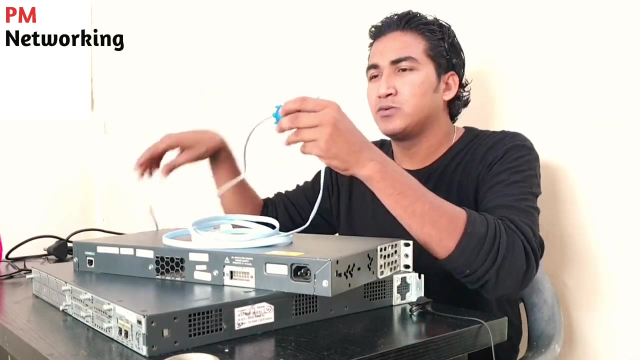 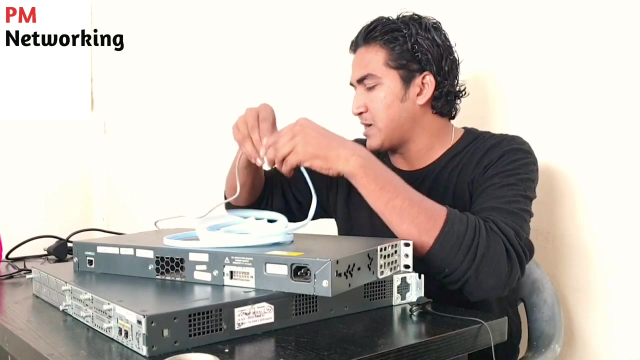 So, but there is no any port. There is no any serial port in my laptop, So we need one more connector, that is, USB to serial connector. USB to serial connector- right? So first we need to connect my console cable to this connector so that I will be able to access, access my devices through laptop right Now. you can see RJ to USB. 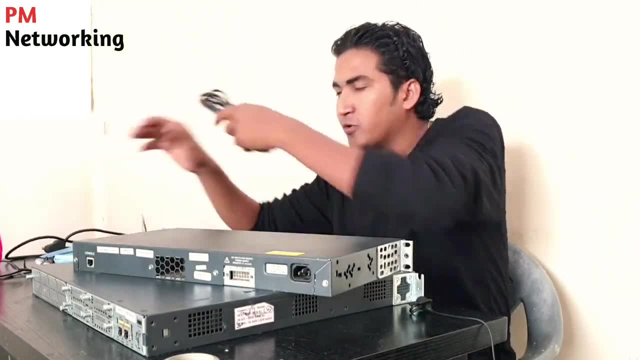 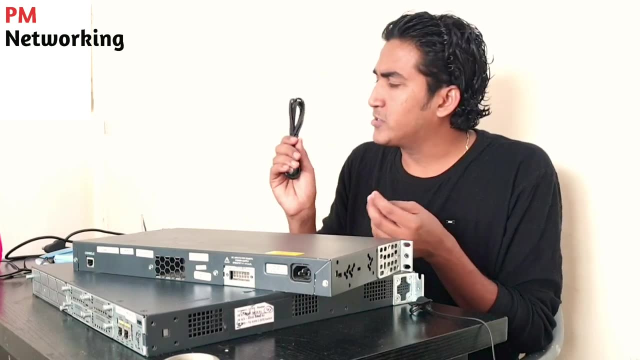 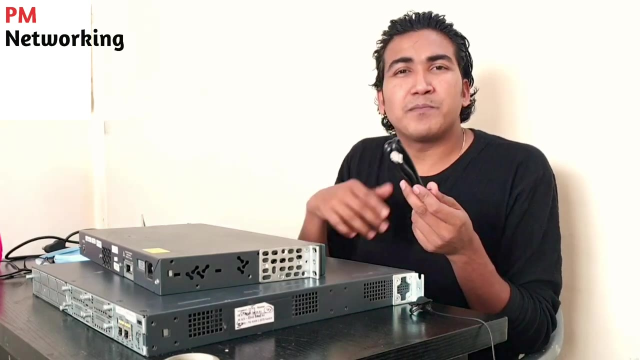 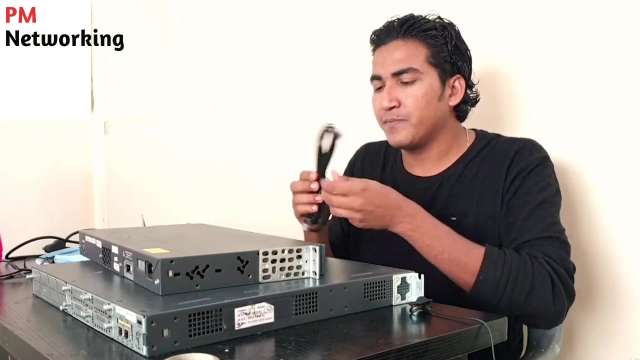 It's fine, It's fine. Let me keep aside for a minute, for a while. And after that we need Ethernet cable, right? So we have multiple Ethernet cable. Don't worry about that, It's. I am showing you just one piece to connect a router to switch, to connect my router to switch and computer through this switch, right, We need Ethernet cable, So it's automatic sensor cable, right? So how we will connect this device together in fast. 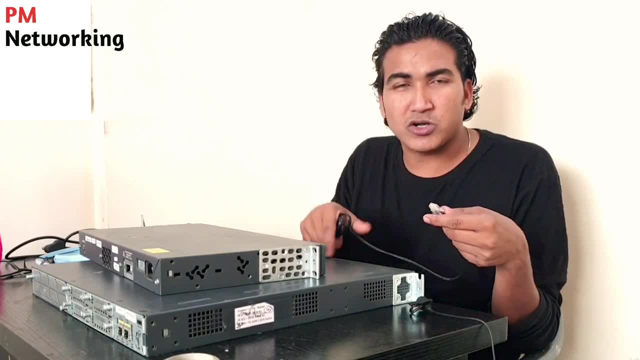 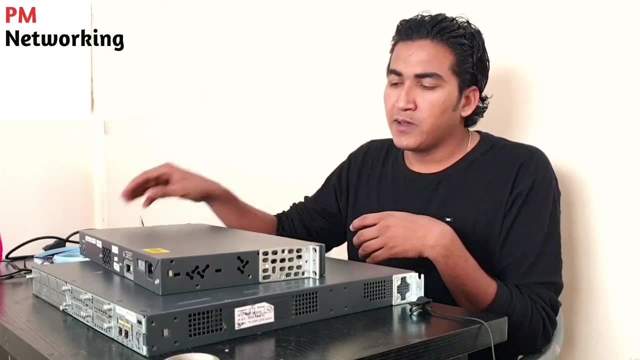 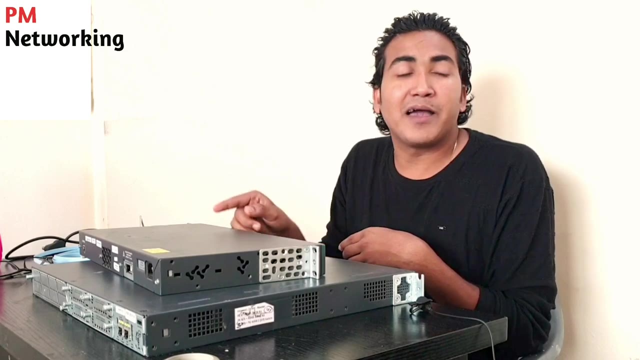 Ethernet 0 slash 0, I will connect to this router on fast Ethernet 0 slash 0 and I will connect one end to this switch right and then I will show you how to connect your computer, my laptop, to this switch and I will enable tel net on router and I will access access my router through this PC through. 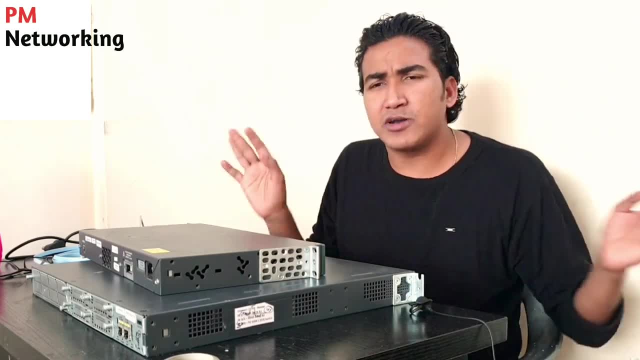 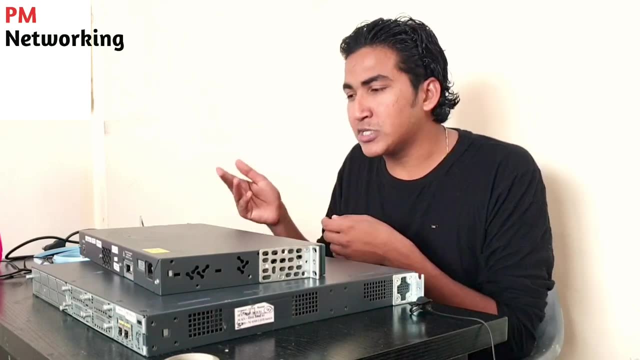 tel and remote access right, So you will see each and everything on your device. Don't worry about that, For today I am going to show you how to access your device right. how to access your device. so what do we need to do first? first, 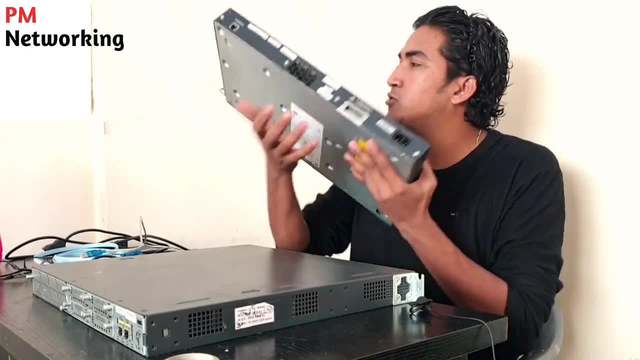 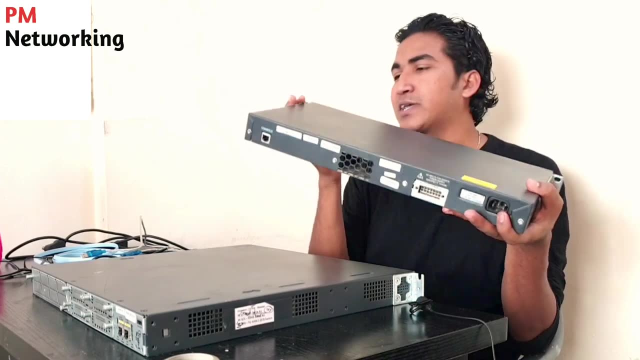 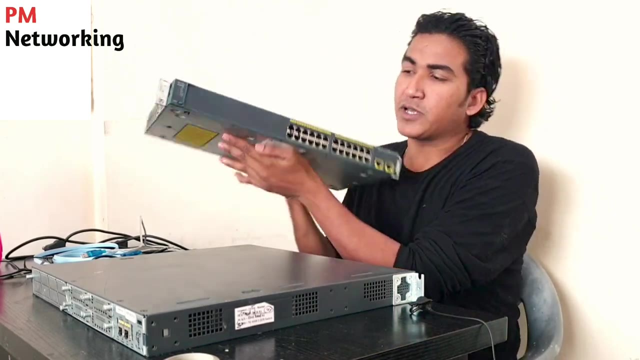 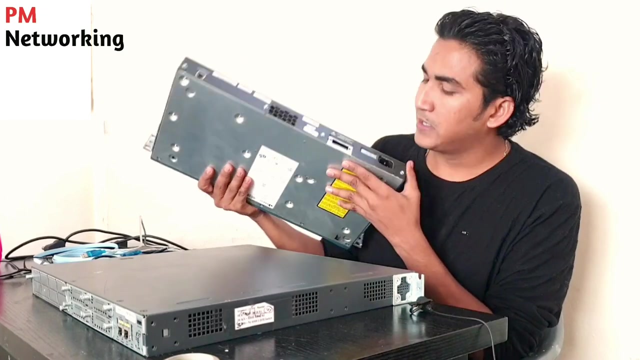 you need to understand about some port. so, guys, as you can see over here, this is my switch, this is my switch. so it is 2960 switch, catalyst, 2960 switch. fine, and we have 24 ports only. i have 24 ports only. i can extend, extend it to 48 ports as well. okay, so just look here. here is one console port. 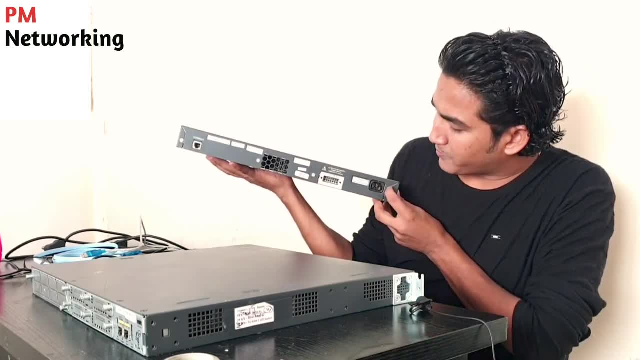 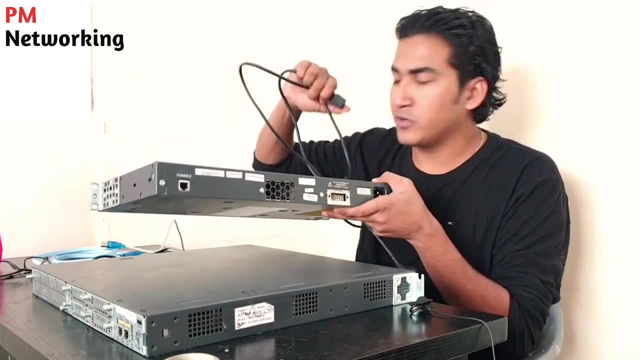 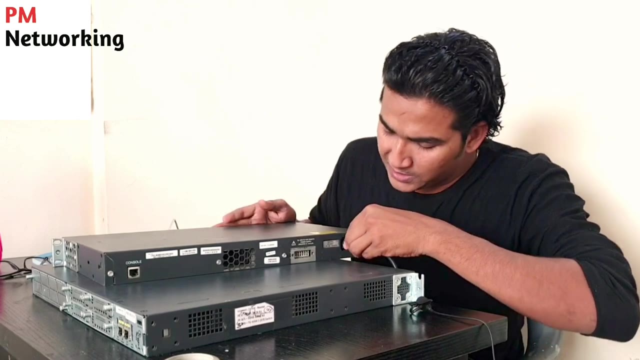 right, you can see, here is one console port and here is one power port. right here is one power port, so you need to connect your power cable to this, this port, right to this port. you need to connect your power cable to this port. okay, and plug this to board. let me plug it. 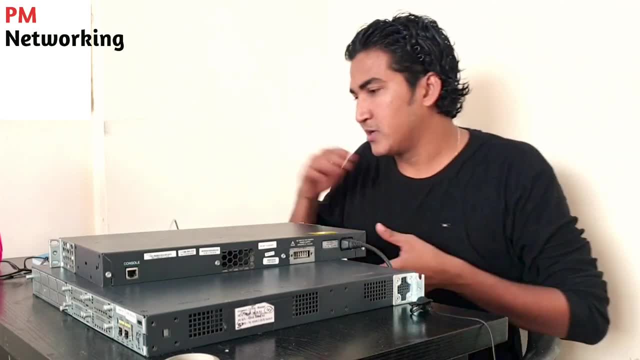 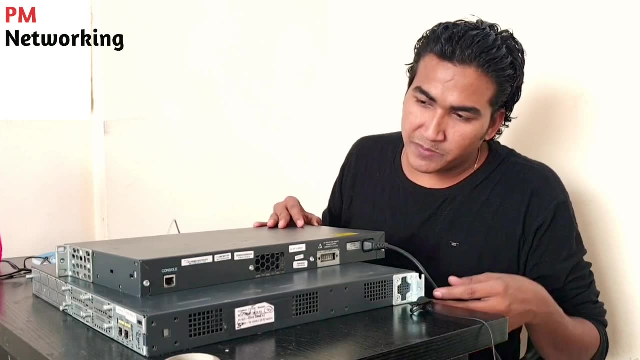 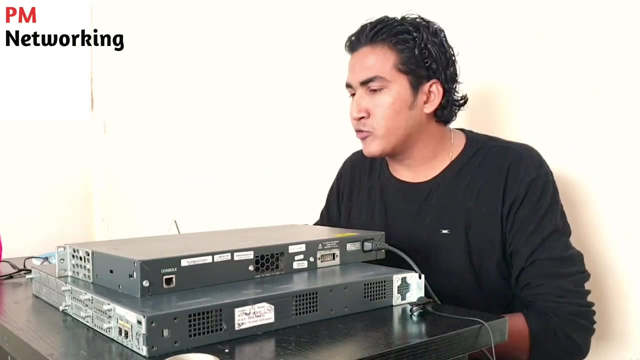 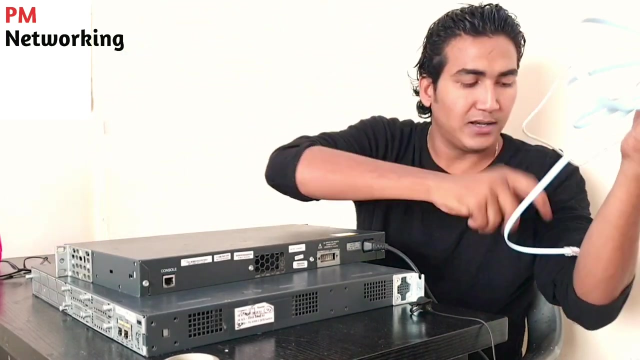 plug it. yes, now my switch is. my switch is on right, my switch is booting right now. just wait for some time. now my switch is fine. what we need to do? you need to connect console cable to this switch console cable. okay, let me connect rj45. 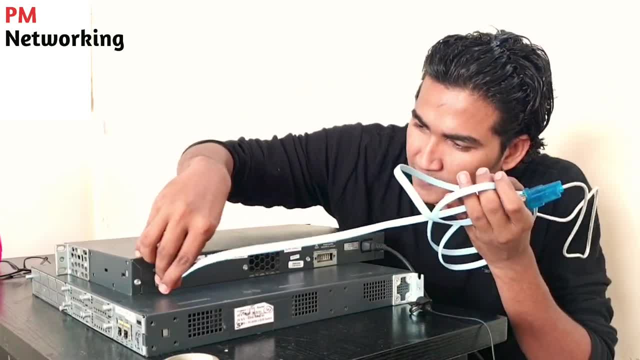 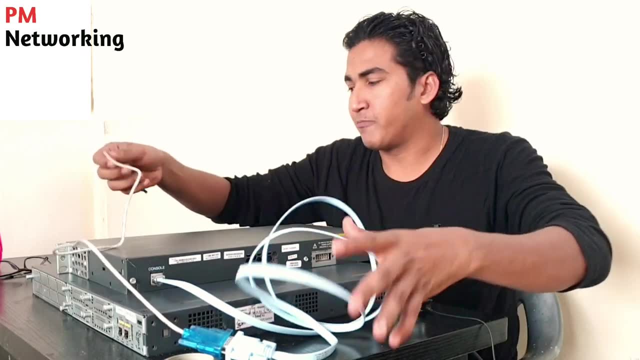 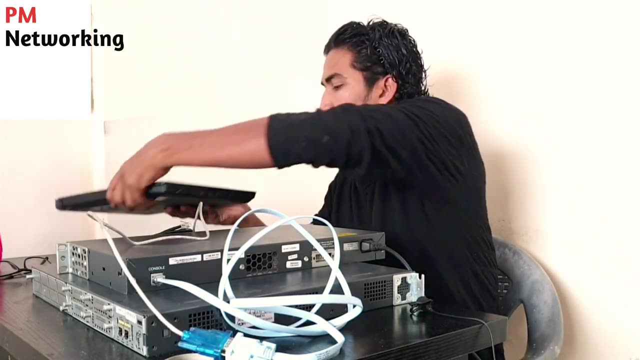 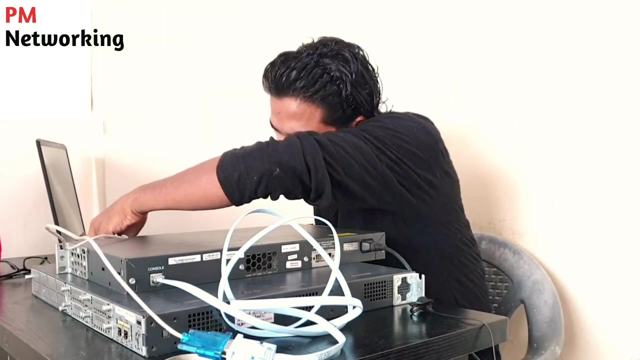 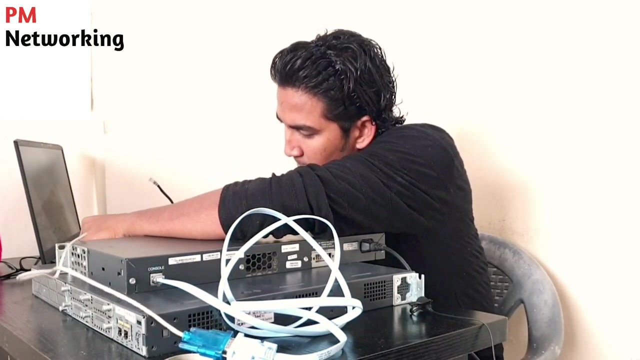 25 console cable of the switch. fine, now we need to connect this USB to my laptop, okay, so, okay, I am taking my laptop over here, over here, okay, and let me connect my laptop through this USB port and let me show you my computer, asking to you. 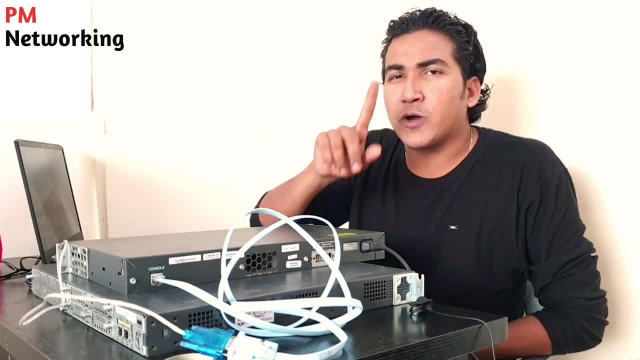 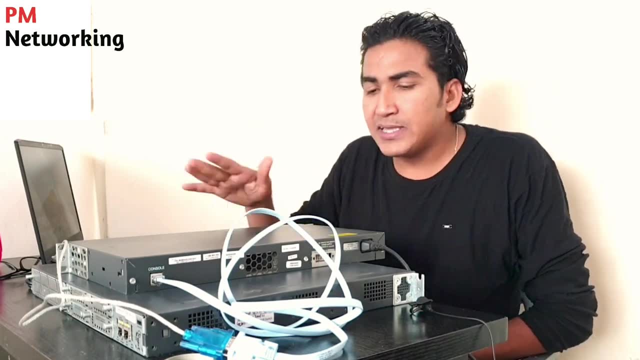 right, it will be more clear to you. you need one software, putty- right. you need to install putty to access this device. right, to access these two device in the same way. I will connect this power cable to router and then I will remove this cable from the switch. 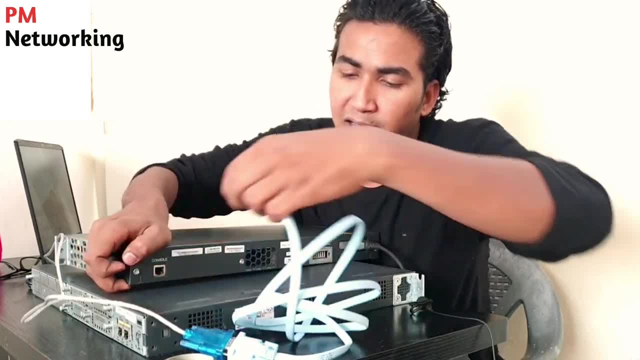 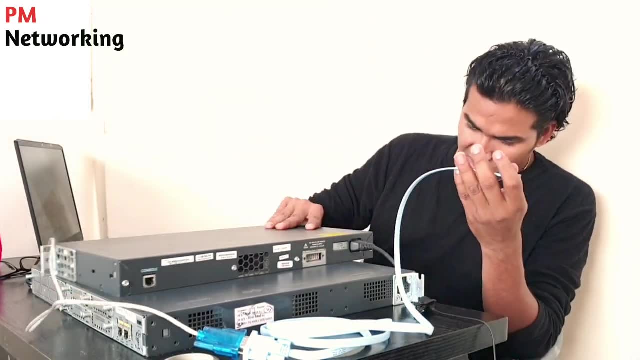 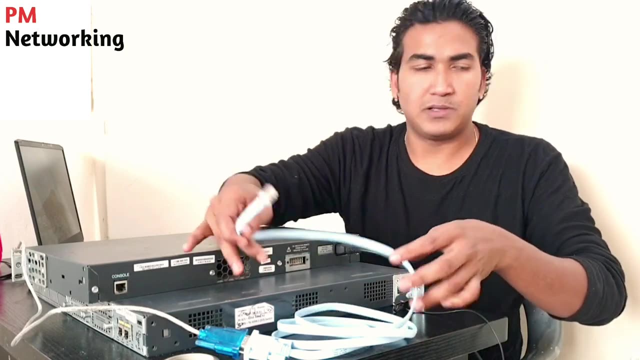 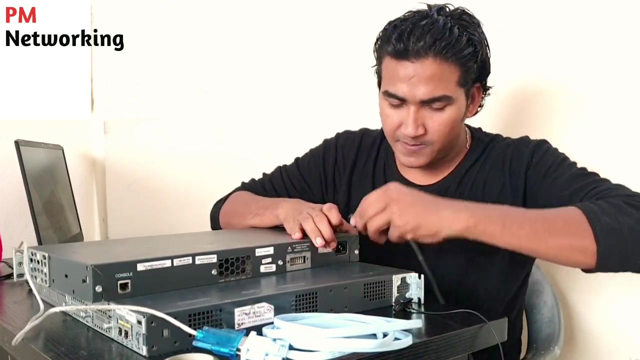 right, I will remove this console cable from the switch and I will connect my router. right, so, router. I also have one console port over here here. right? okay, here is console port. let me show you router first. let me disconnect it. disconnect it- okay, how router looks. okay how router looks. 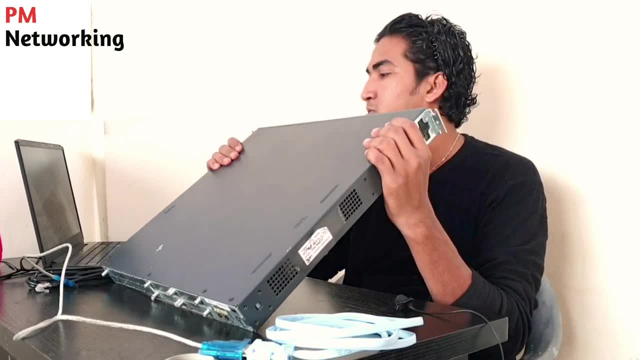 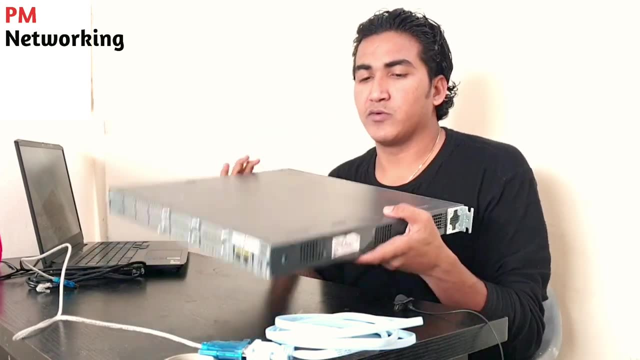 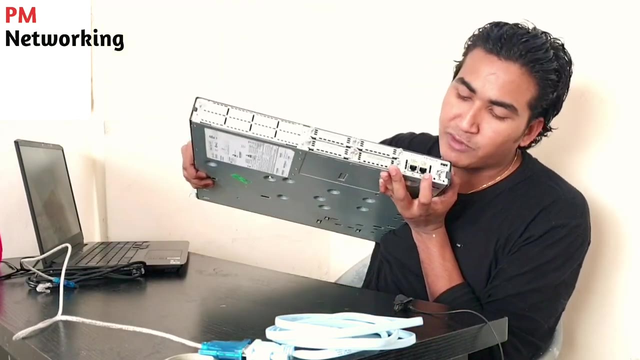 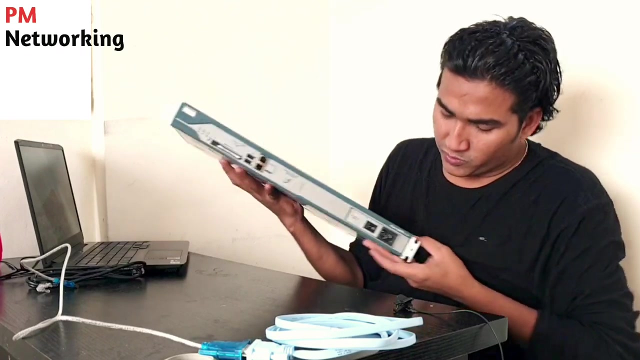 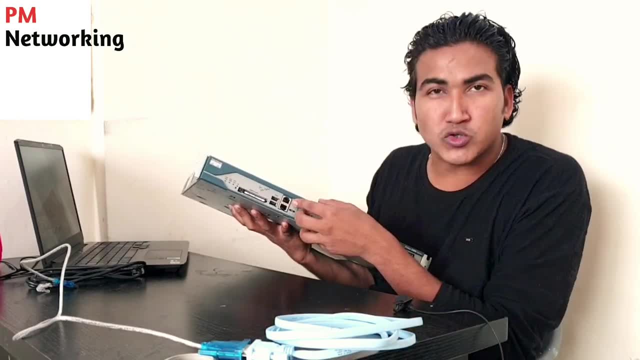 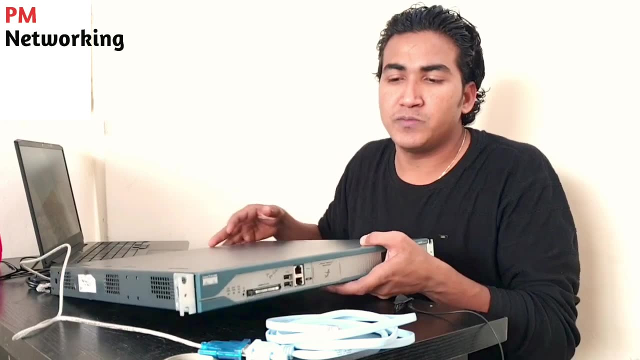 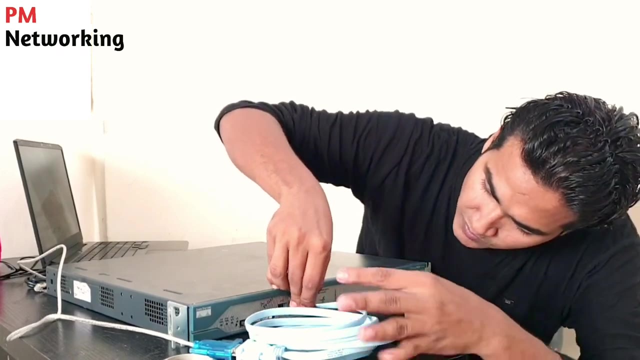 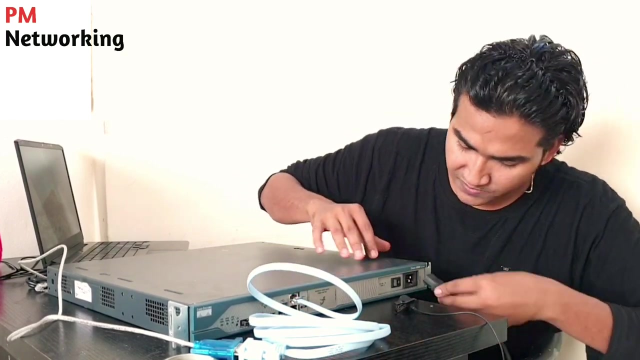 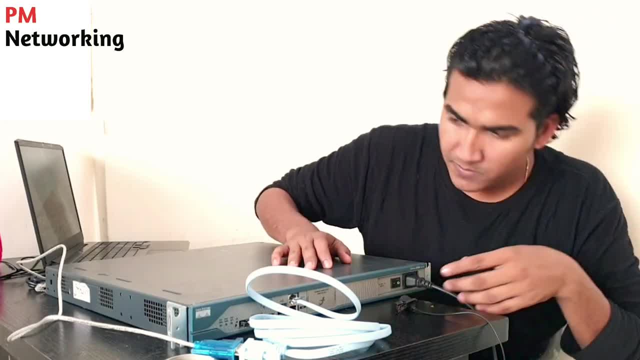 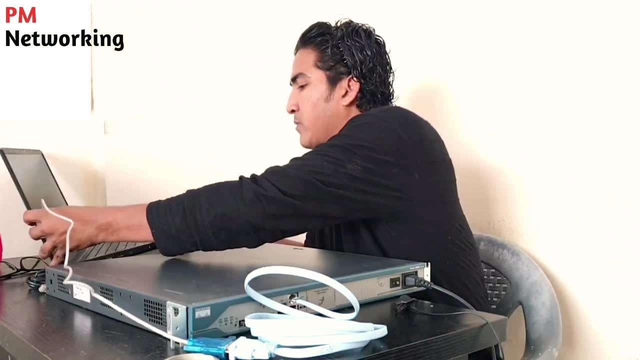 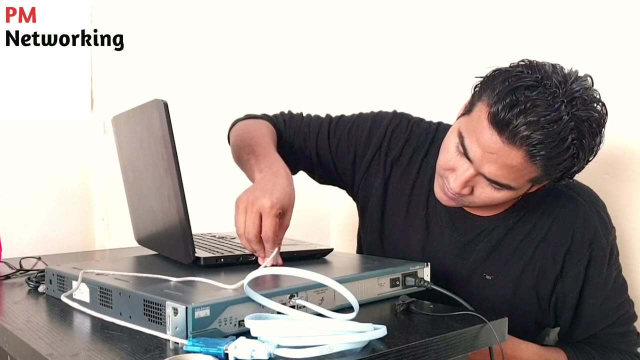 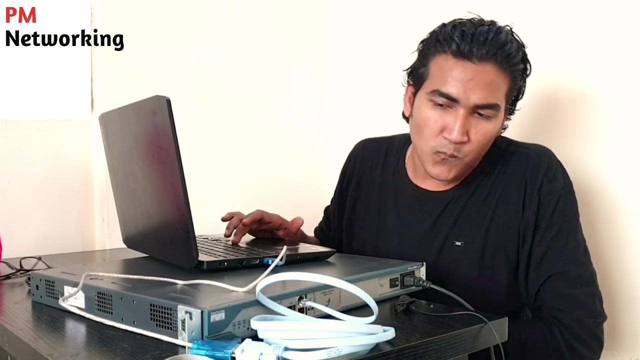 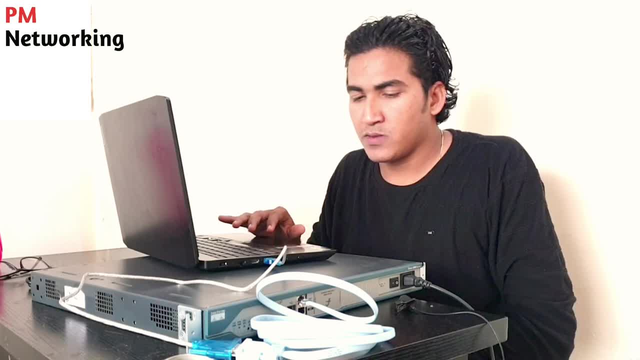 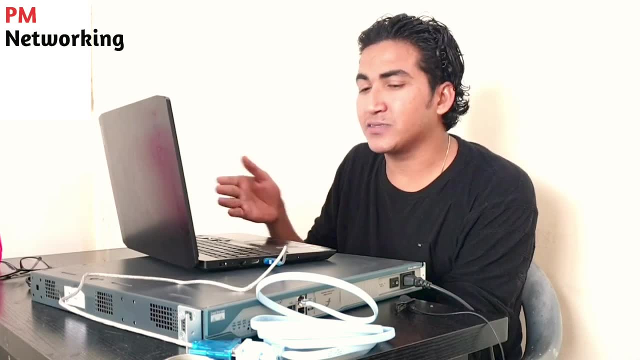 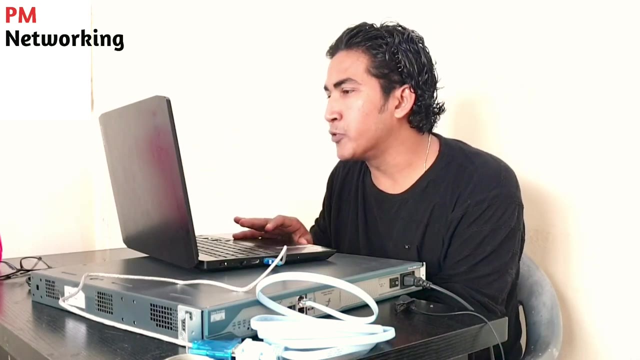 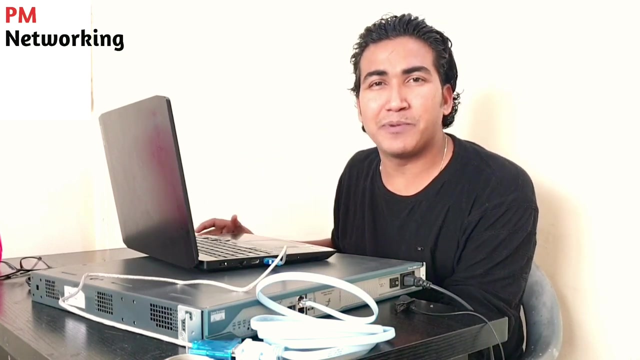 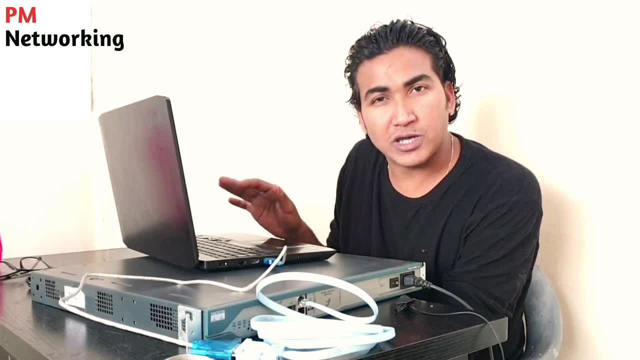 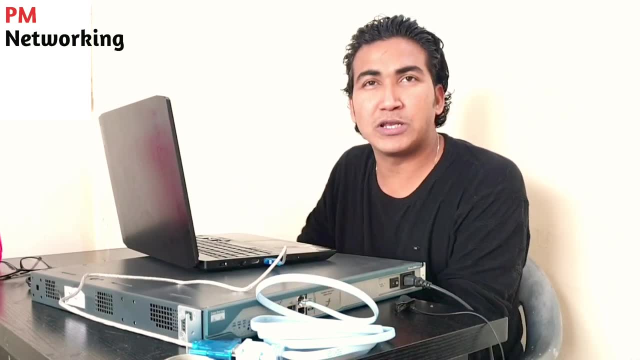 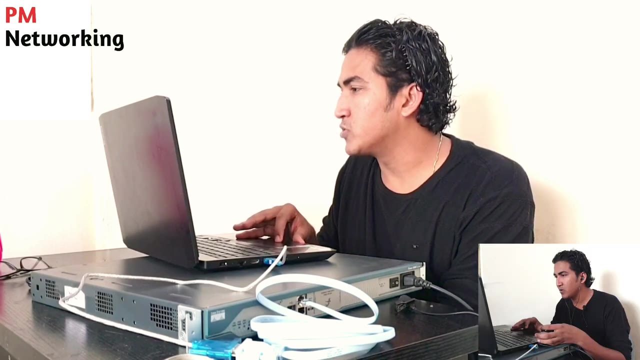 this router in the same way i am accessing right now. okay, you need to connect your console cable on console port and one port in your laptop. now. router is booted right now. let me. let me show you my computer screen first to you. okay, so what we need to do over here is we need to open putty. 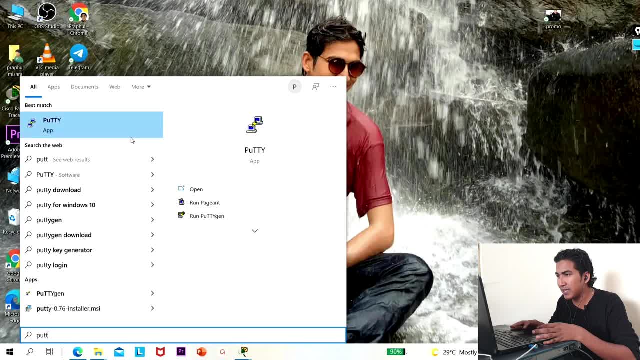 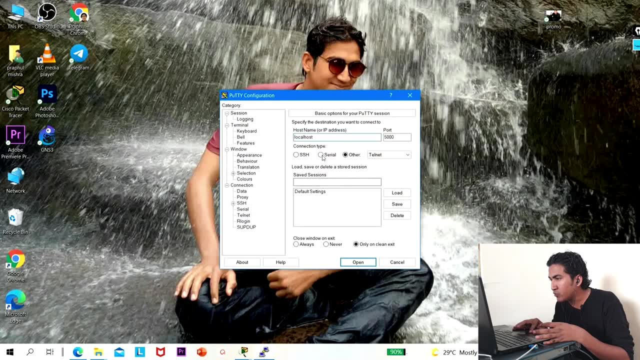 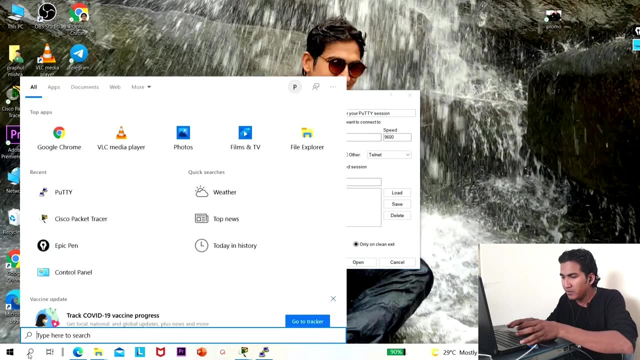 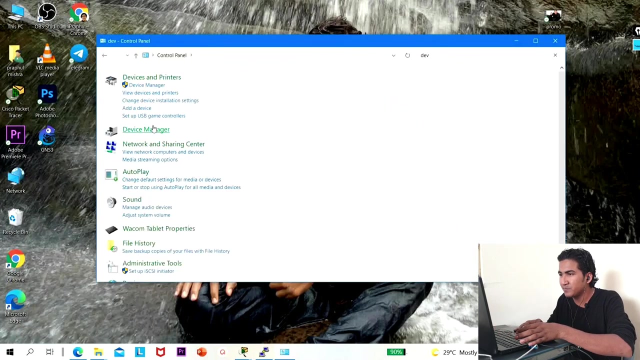 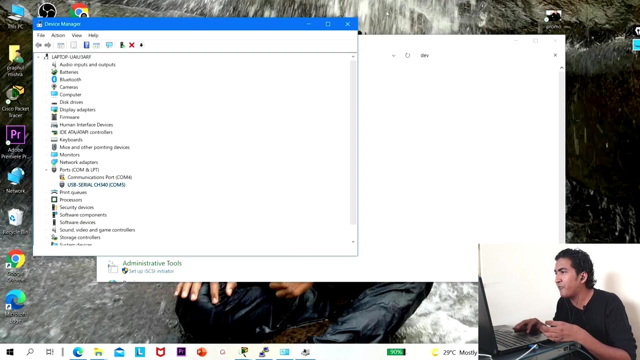 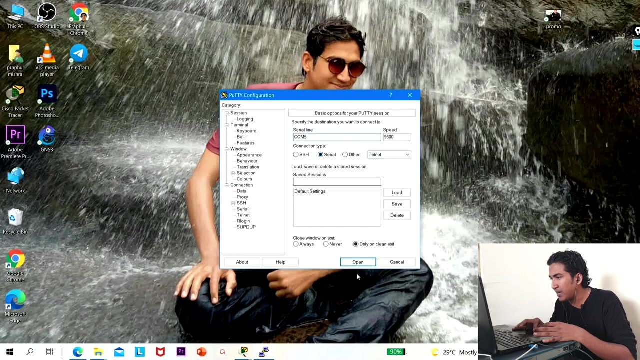 so putty, click here. run as administrator. yes, okay, guys, see, here is one serial option, so click on it. serial option, not serial line. let me check my port number. so go to control panel. go to control panel, then device manager, device manager and port number. serial port number is com 5, com 5. okay, let's write com 5, click on serial and open it, just wait. 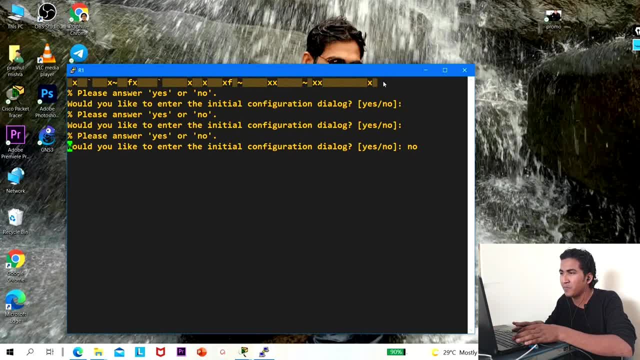 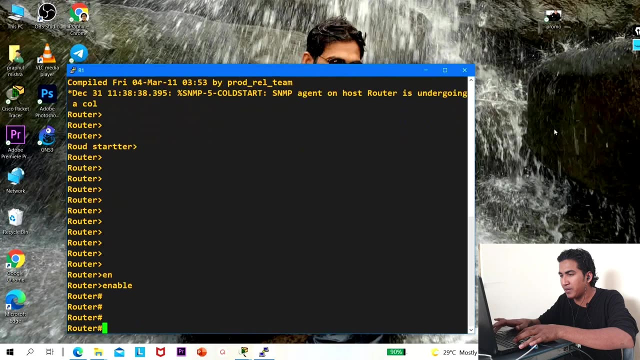 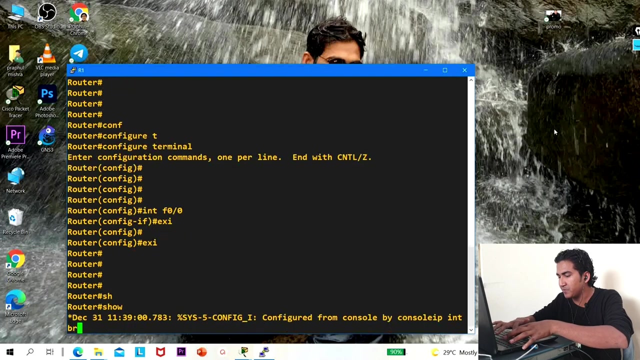 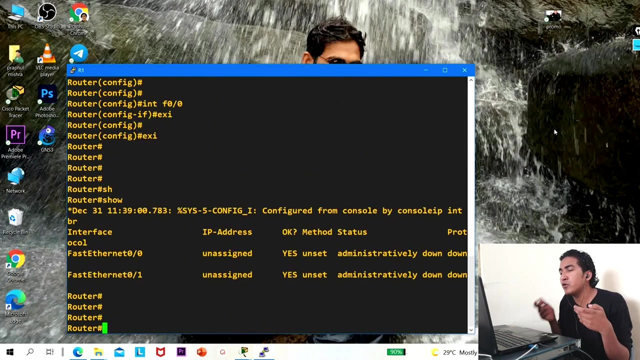 no, and you can see i have access of router right now. okay, now, i'm now running your business computer right now, so i am running building computer. okay, anduku, now i'm somewhat in the starting mode of langa, so, yes, i'm running. enable terminal interface: fast ethernet: zero slash, zero exit, exit. show ip interface brief.